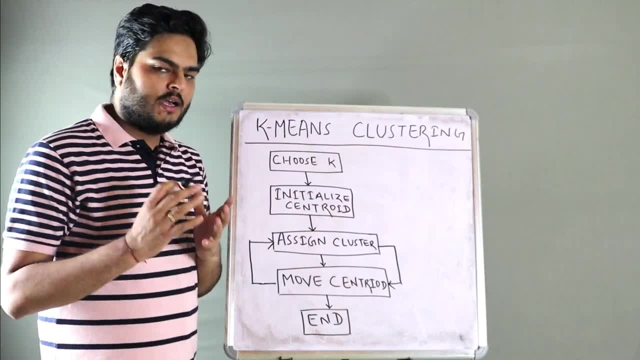 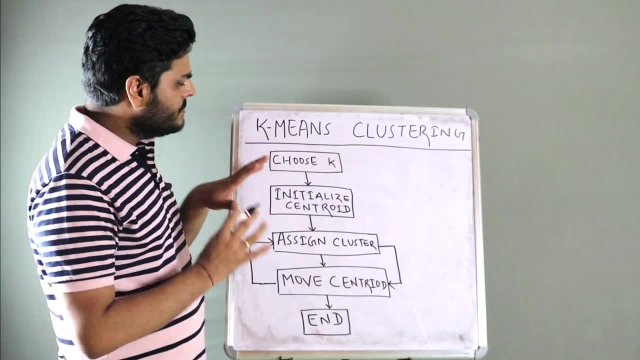 welcome to unfold data science friends. my name is aman and i am a data scientist. in next 10 minutes i am going to explain you k-means clustering in a very simple and easy way. i am going to tell you stepwise process of what happens in k-means clustering. 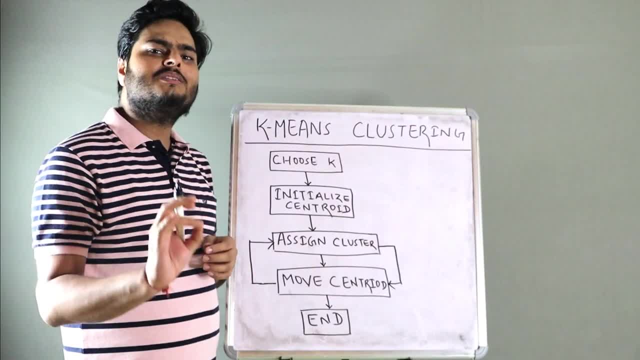 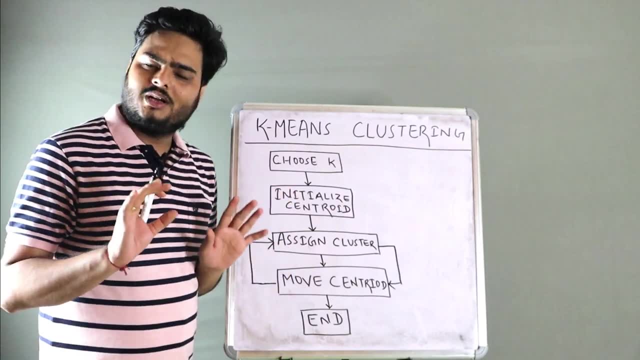 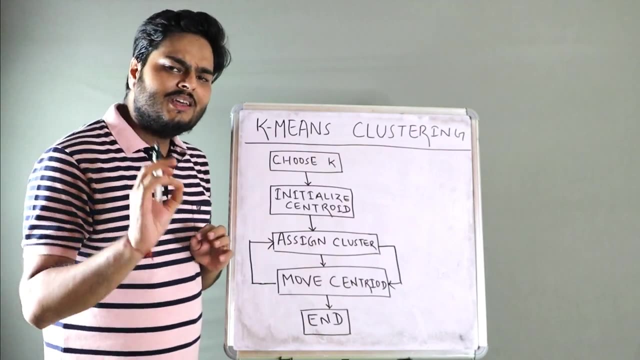 and also going to show you in python how to implement a simple k-means clustering. okay, if you watch this video till end this topic, you will not forget easily, that i can assure you. okay, let's start, guys. what is k-means? k-means is nothing but a technique to cluster what is. 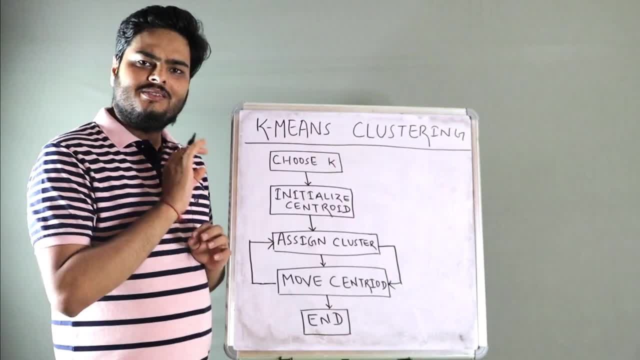 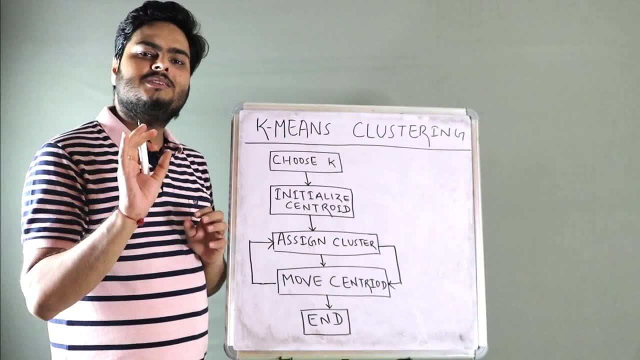 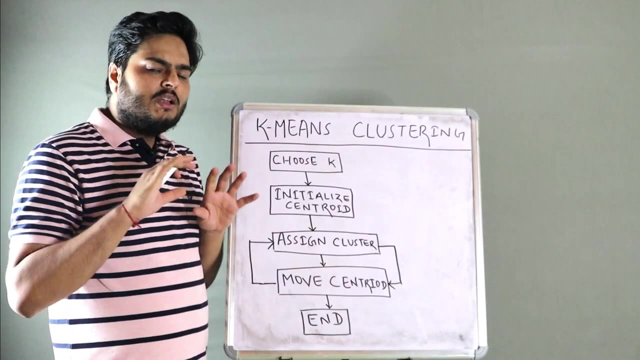 clustering. i had created a detailed video. the link is here. you can watch this. clustering is nothing but grouping similar things together. those similar things can be customers, products, websites, anything which has certain features and attributes right now. when we want to group similar things, then we will consider its attributes right. 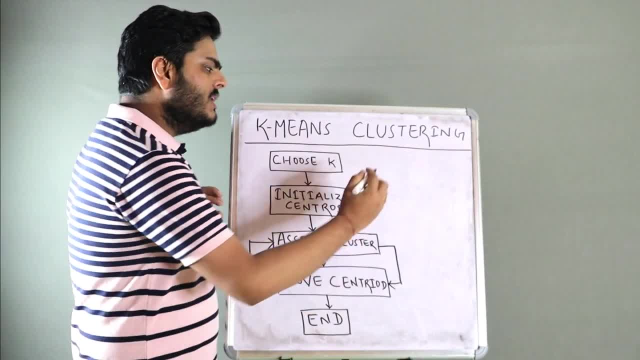 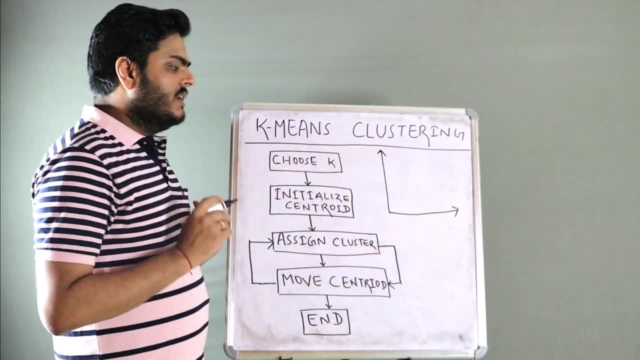 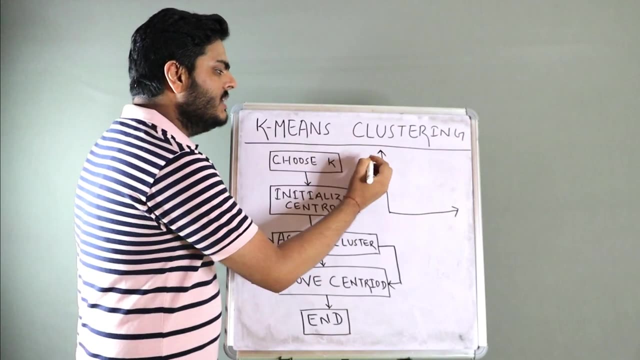 so what i am going to do here is i am going to create a simple xy chart first. okay, i'll come to this side of the board later. simple xy chart. in this chart i am going to put income and expense of people. okay. for example, here i am putting expense and here i am putting income. okay now. 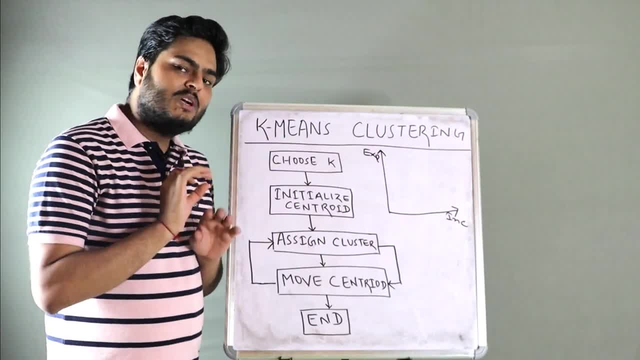 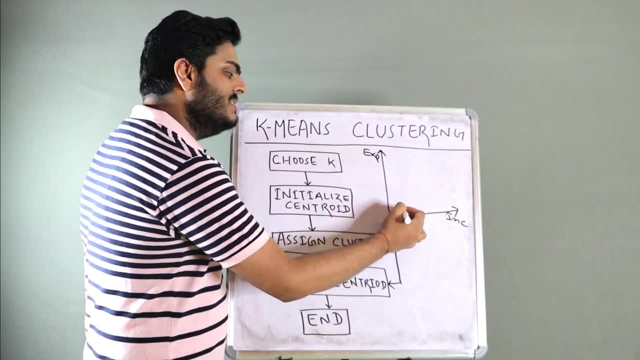 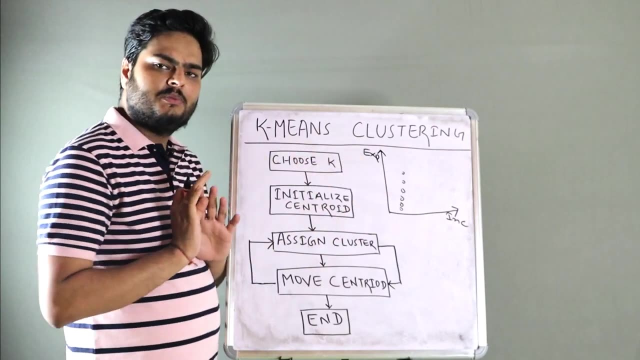 there might be people who might be earning less but spending little higher. okay, let us assume there are some people like this, so their income is lower, let's say in this range, and their expense is, you know, little higher side. some people- not everyone, but some people. on the other hand, there are people whose income is more, which means they will be somewhere. 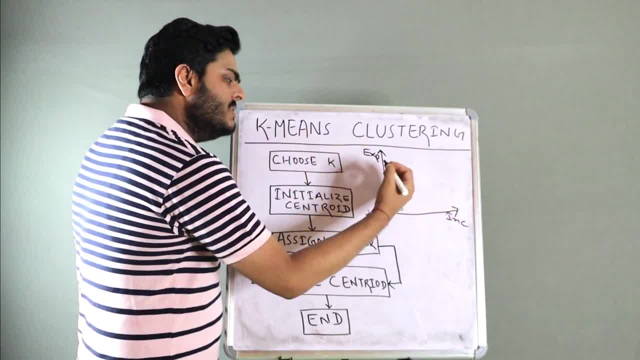 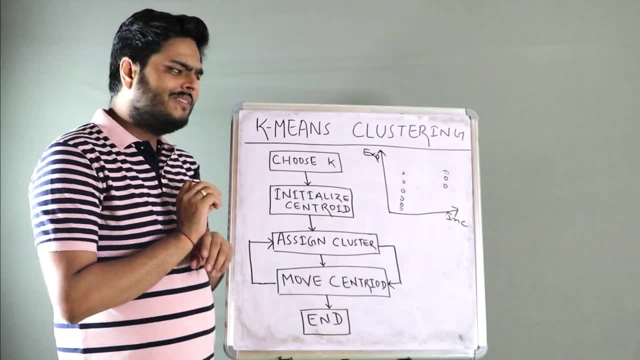 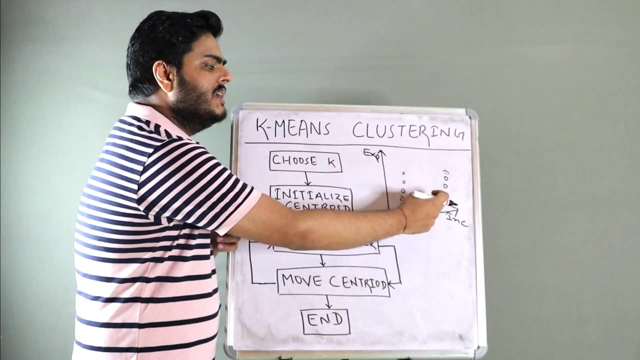 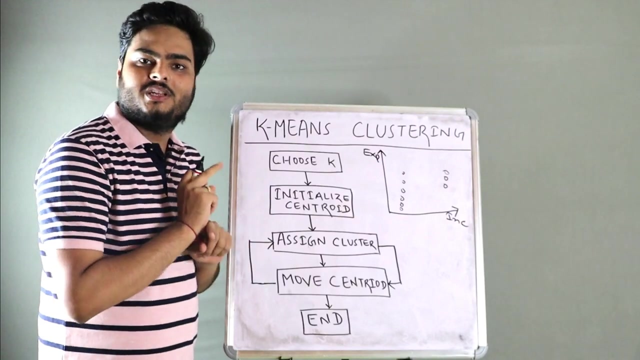 this side and their expenses, you know, similar to these guys, so i can say something like this: not too different from these guys. what i am coming here to say is these guys are aggressive spenders. even if they earn less, they spend more. these guys, even when they earn more, they are spending. similar to these guys, only so there is a behavioral difference. 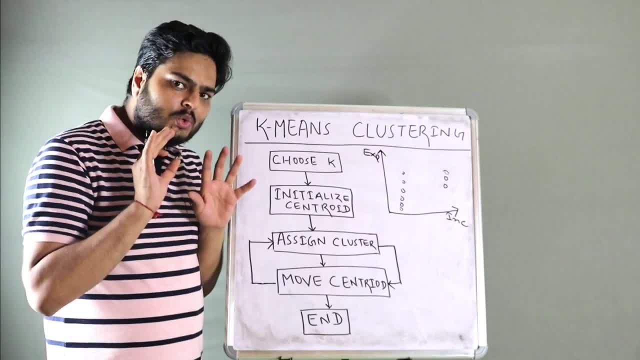 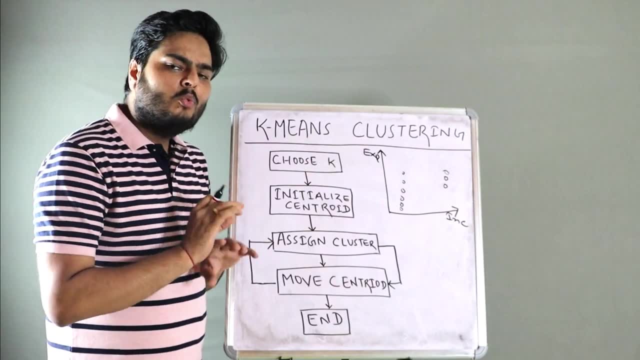 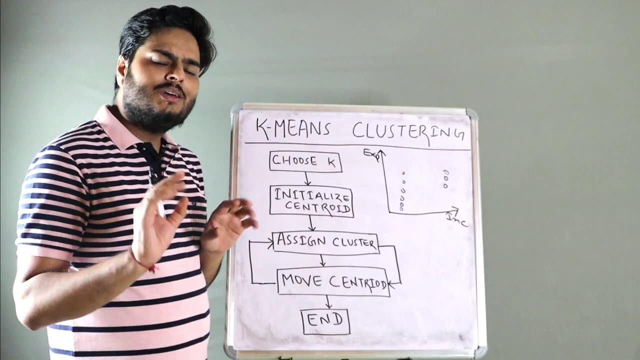 and that is what we intend to do in clustering. we want to understand the behavior of different customers. in this case, let's say customers. now, what we will do is: we will understand when we take this and submit it to k means in the public. it means that we can know the organization of the business when it comes to 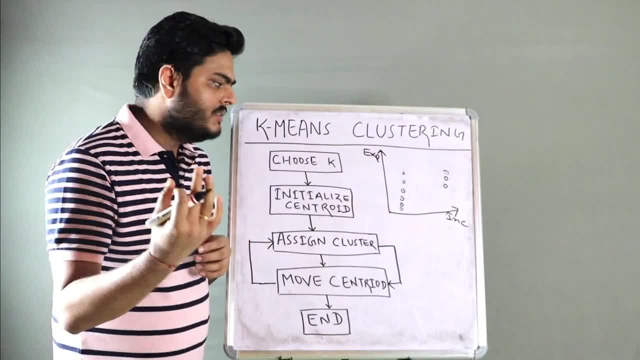 everything and, in the end, correct me if you just listen carefully. what i want to do is when i inviting these people and one of these people, i will do such a, so it will just let them know how they should discuss. i just needed to watch to see how many people they want right now. 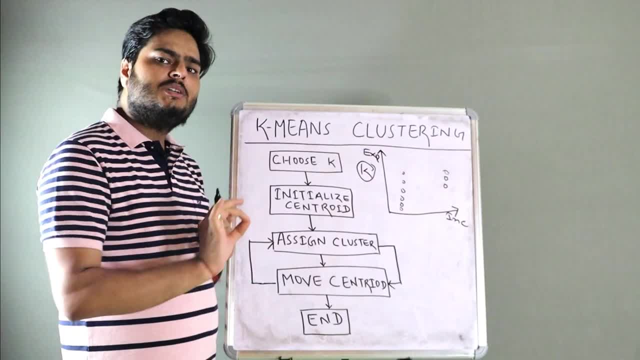 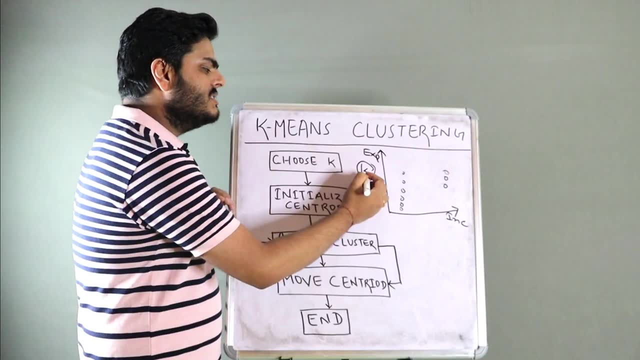 so when you look closer you will see. you can see in the beginning the store or the next store and you can see that the store再見 is planning first in june is closing, like this is in june. so then you might notice- after all we have said that everything is looking okay- the whole industry in 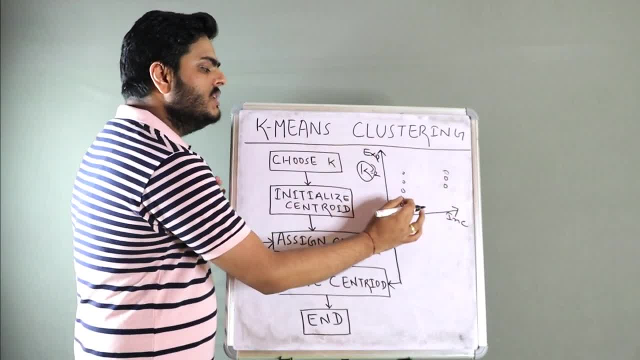 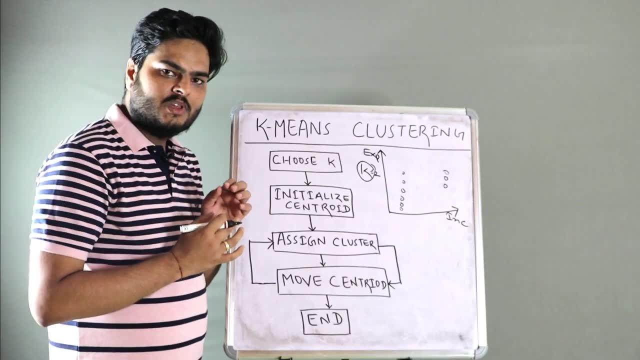 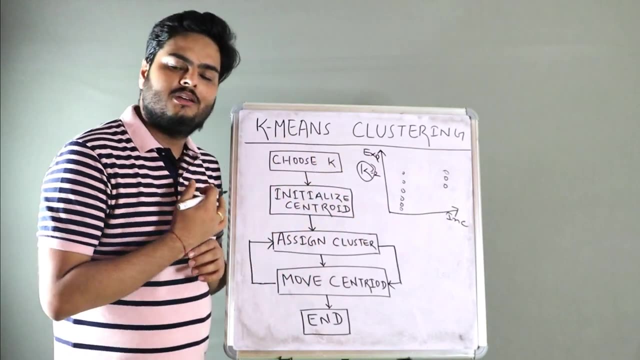 kind of behave similarly. one is this group, one is this group. one is, you know, not very aggressive spenders. one is aggressive spenders, let us say, in our case, k is two. this is the step number one. what happens next is initialize the cluster centroid. what is cluster centroid, guys? so when i 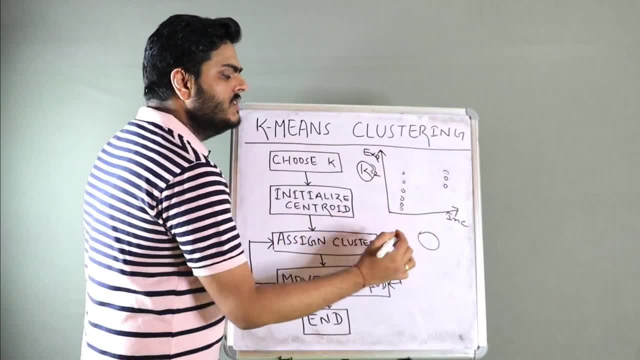 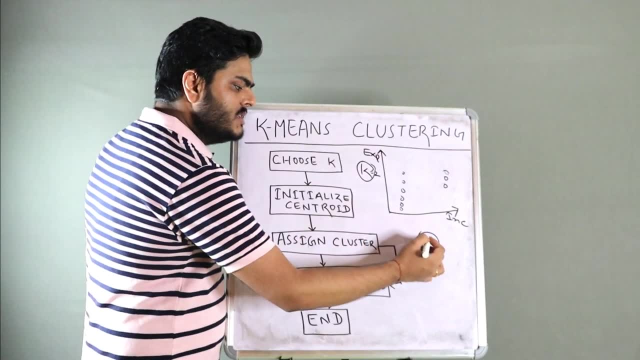 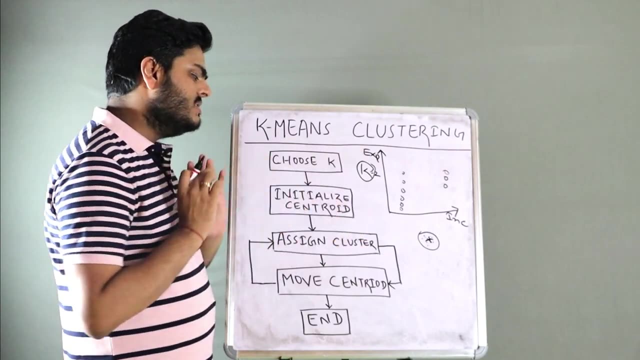 say: this is my one cluster, which means there are many people in this cluster. right, so there will be a central point of this cluster. you can say this as a central point of this cluster. that is nothing but centroid. okay, so what will happen as a next stage is the python will initialize two random 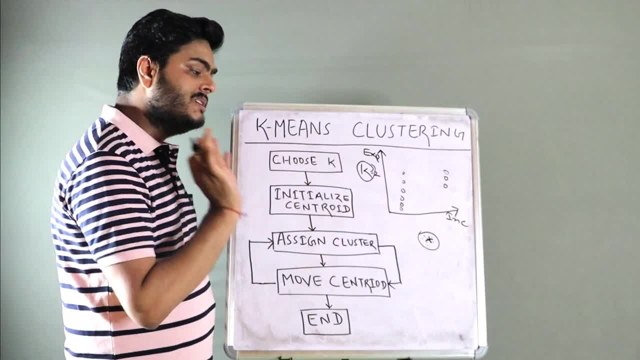 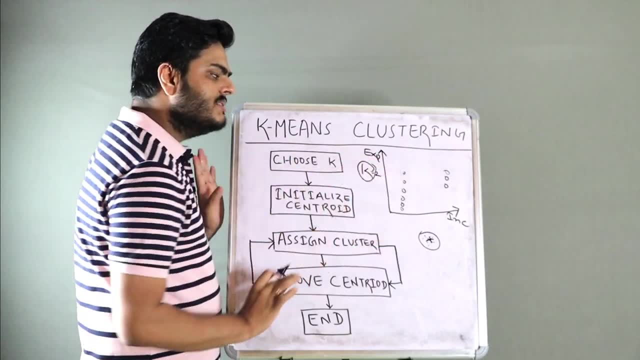 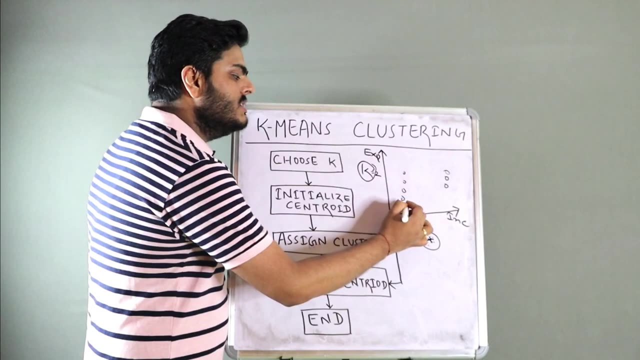 centroids, okay, random centroids from the data itself. if you say one argument is there, if you say random, then it will take random data points from these and think this is the cluster centroid. let us assume, for simplicity, this data point is randomly initialized centroid for cluster one and this data point is randomly. 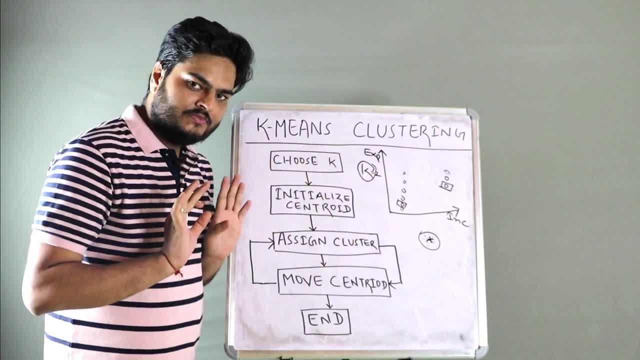 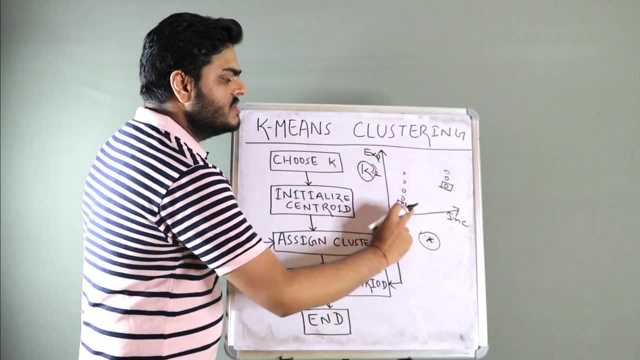 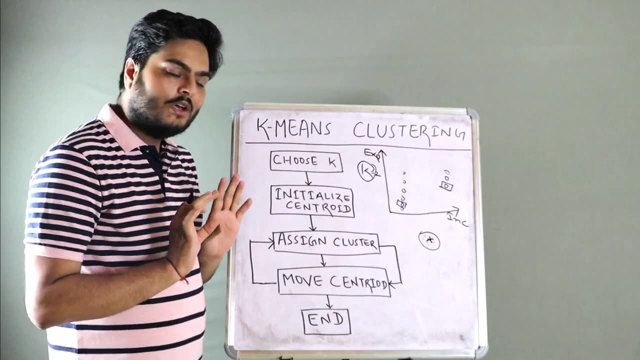 initialized centroid for cluster two. clear up to here, this is step number two done. now what will happen is all the data points. all the data points will be seen for the assignment. okay, now we have how many data points? one, two, three, four, five, six, seven, including the centroid. 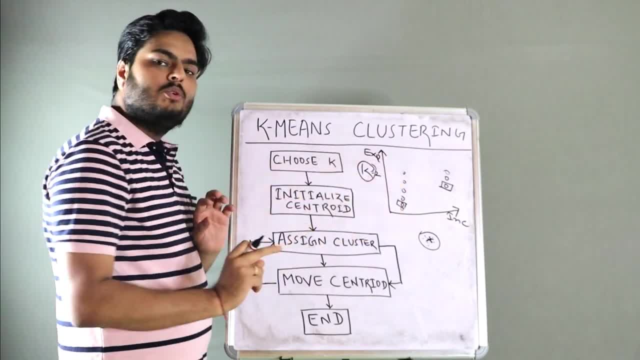 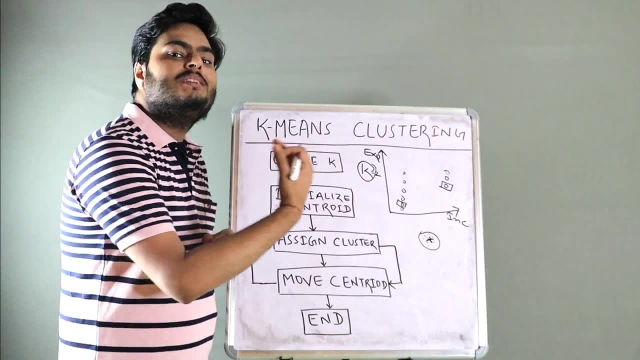 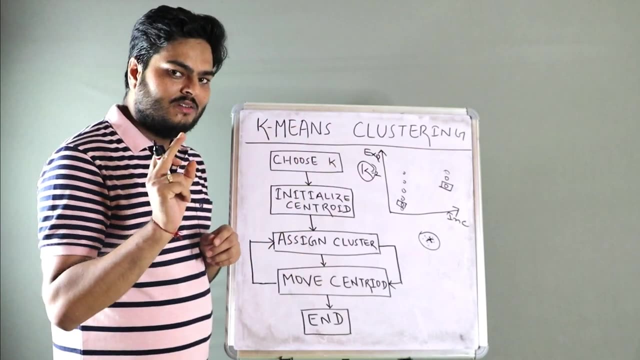 one, two, three, ten data points. all these data points will be assigned to one of these centroids. which centroid whichever is near what is near? in this case, i had created a detailed video on different distance matrices. the link is here. you can watch. in this case, you can consider the. 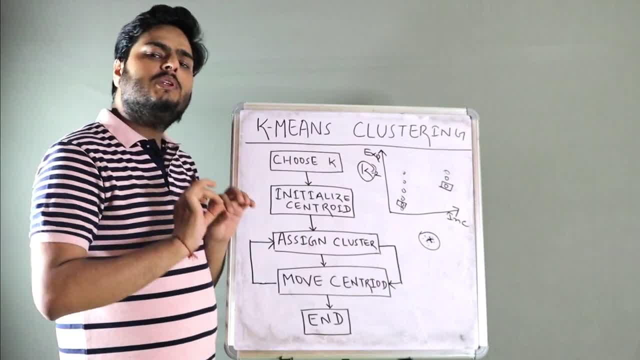 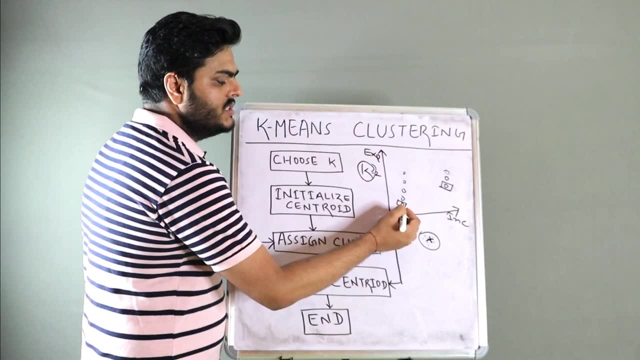 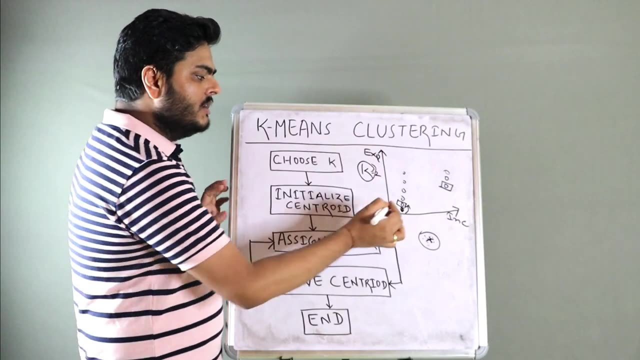 euclidean distance. when i say near or far euclidean distance, you can consider: okay, so this point is this centroid. so this point, for example, is it closer to this centroid or this centroid? obviously this centroid, so assigned to this. fine, this point is it closer to this centroid or this? 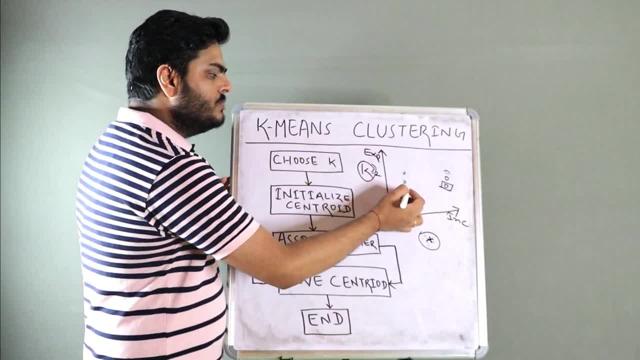 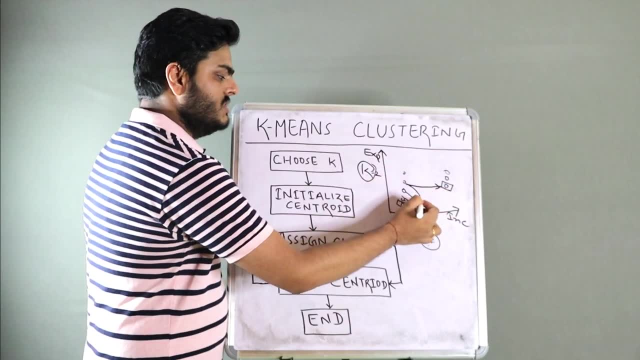 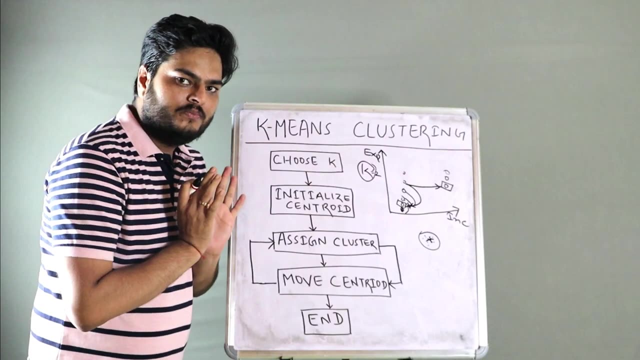 centroid, this one, so assigned to this cluster, this point closer to this one, or this one, this one, this point, we do not know. it can be closer to this also, or this also, we do not know. whichever is closer in euclidean distance, it will be assigned. one assignment is complete. what? 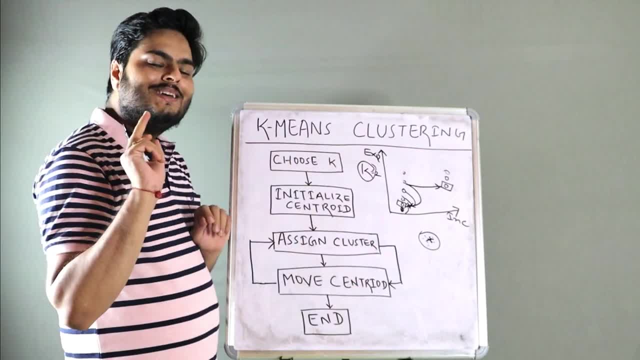 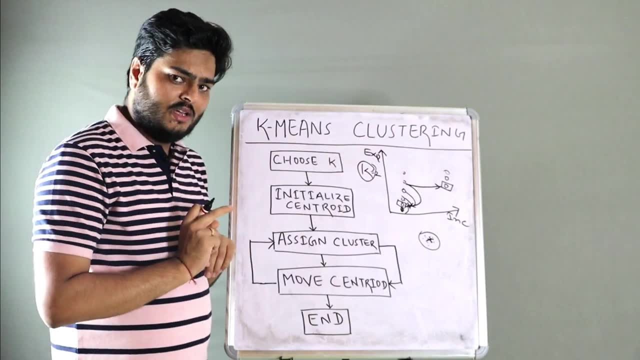 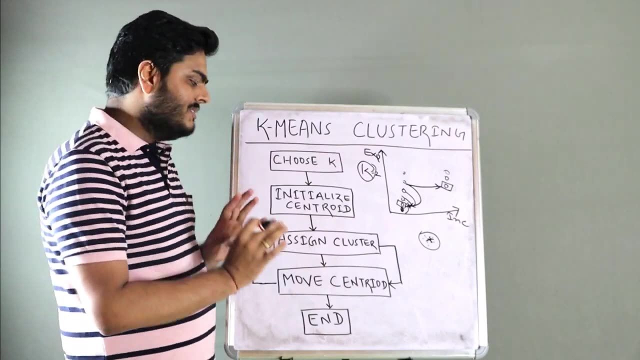 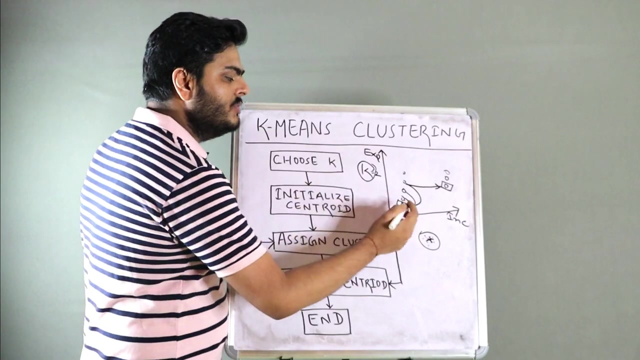 happens next is after assigned clusters, the new centroids will be computed. this is very important to understand, guys. what is new centroid here? imagine, understand the first centroids were randomly initialized, but the next centroids will not be randomly initialized. it will be a mean of all the data points in this cluster. for example, if i say that these three points are: 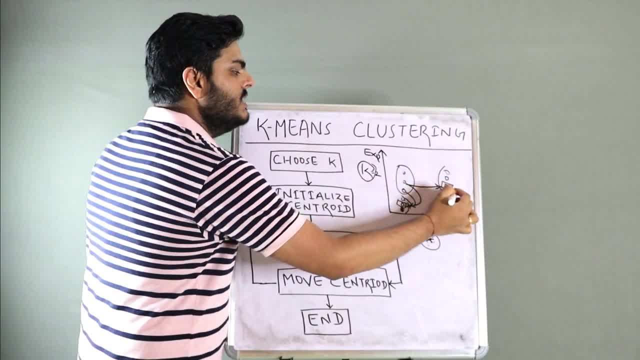 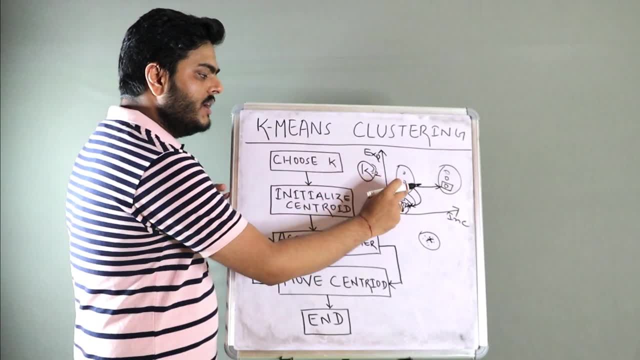 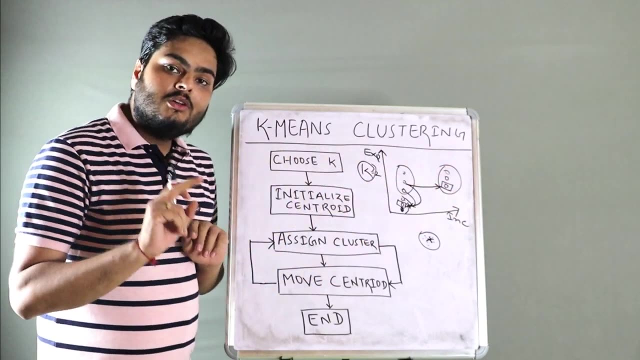 in cluster one, just for example. i'm saying: and these three points are in cluster two, then the mean of all the x values and mean of all the y values, that becomes the new cluster centroid. the mean of all the x values, mean of all the y values, that becomes new cluster centroid for. 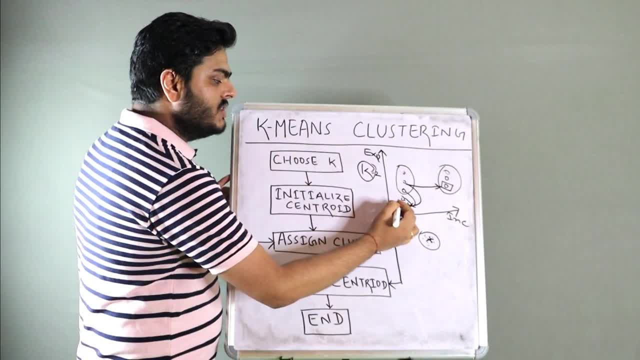 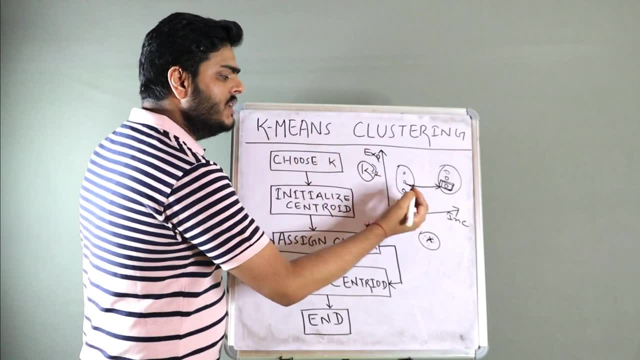 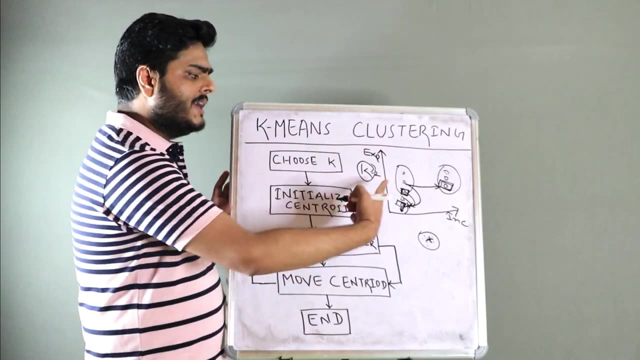 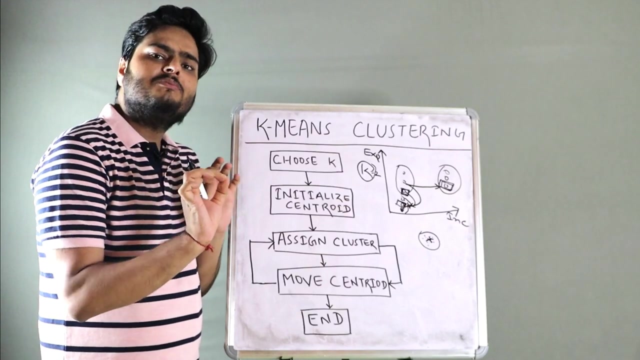 cluster two. now we started from this centroid, but in the iteration two we got a new centroid. let us say that new centroid is somewhere here, or this point is this centroid. now what happens, guys? again assign cluster, how again see the distances of all these points from both the centroid, whichever is near assigned to that? so there will be some shift, there will be. 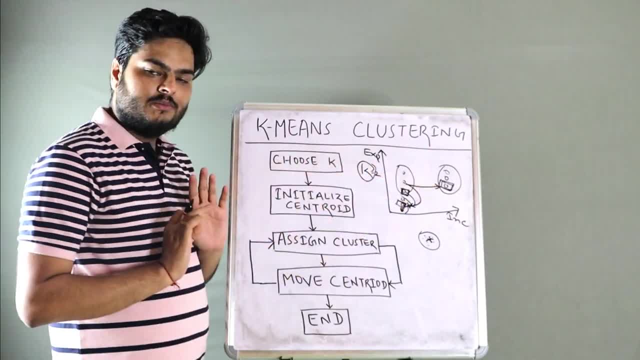 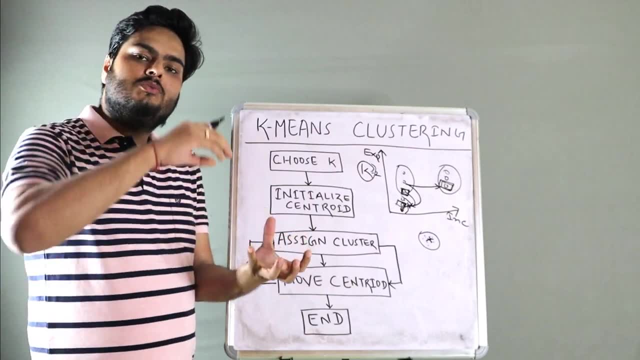 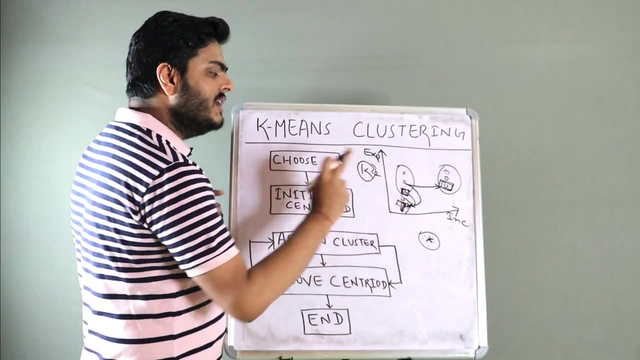 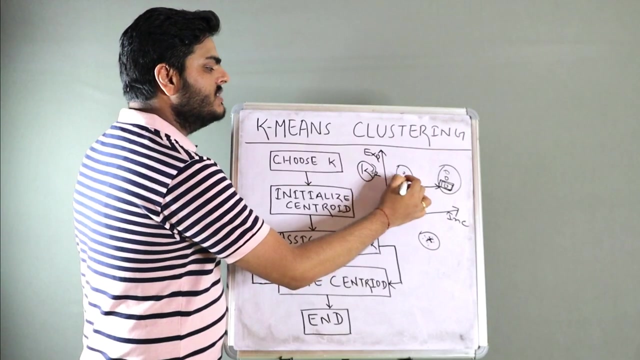 some points which will move from one cluster to other cluster. okay, and then centroid will change again. how take the mean of all the points in one particular cluster that becomes the new centroid, and iteration three starts every time centroid is shifting. one iteration is getting completed, okay, iteration one. iteration two: centroid shift, attrition three. there will be a point where it 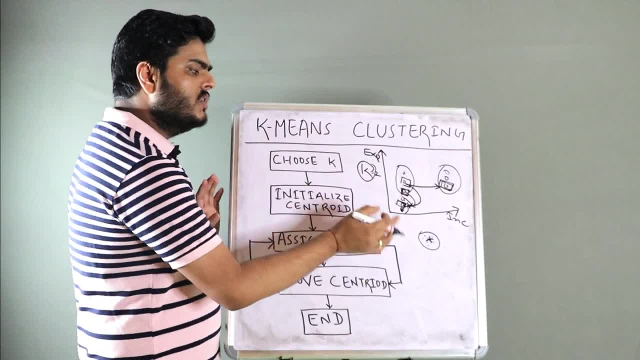 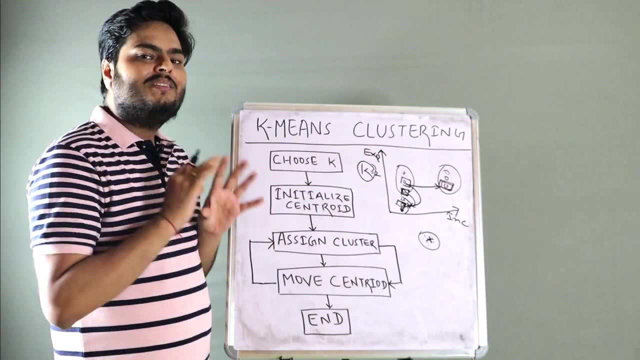 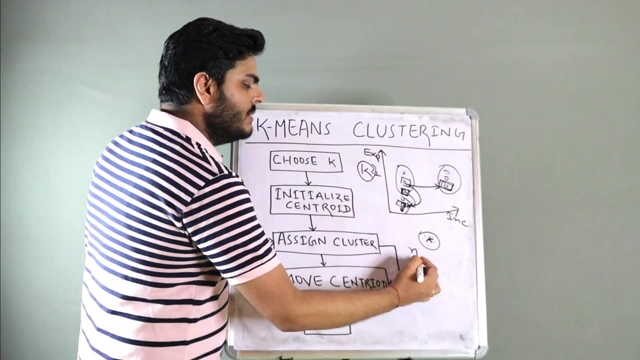 will be no shift in the centroid, which means new centroid and old centroid will be same, and that is where your clustering algorithm converges, or it says that these are the final clusters. in case of centroid, you can give a parameter called number of iteration is equal to, let's say, 300, then the 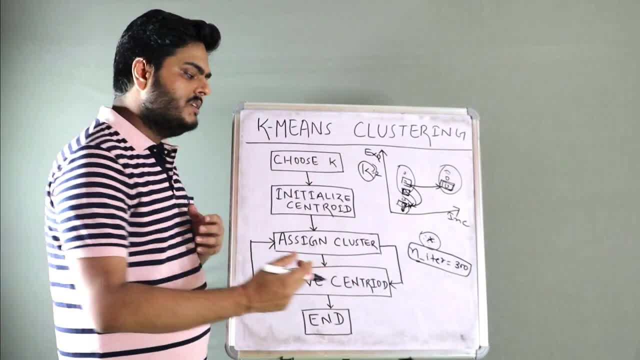 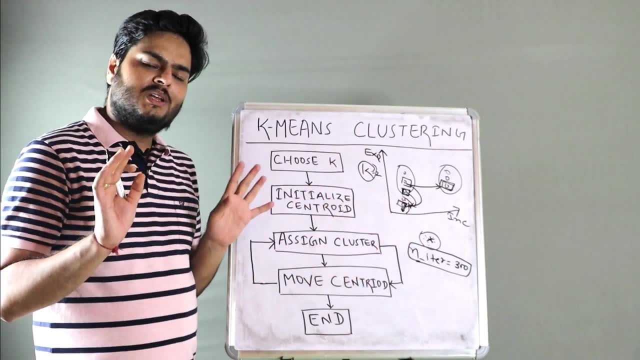 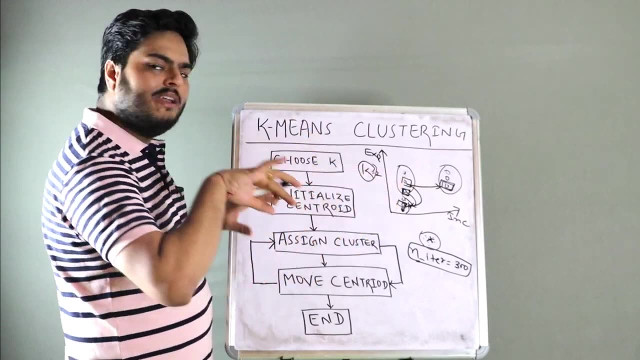 centroid shift will not happen more than 300 times. okay, that is a parameter you can pass, but it will automatically converge before that, only if you have a simpler kind of data. okay, so this is how: choosing k, initializing centroid, assigning the data points to those centroid, calculating mean for. 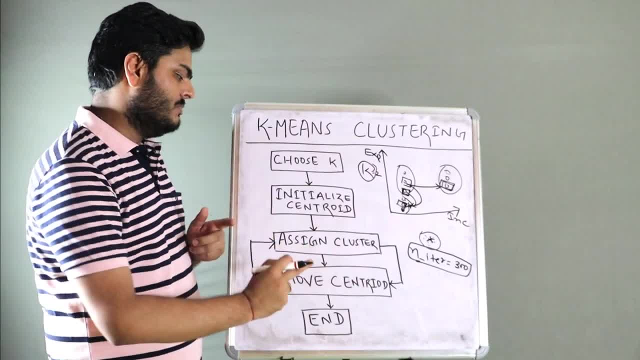 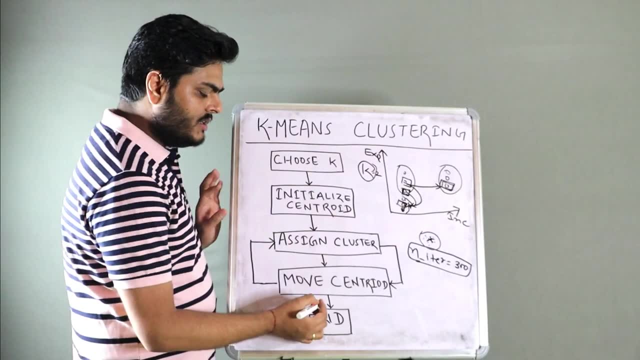 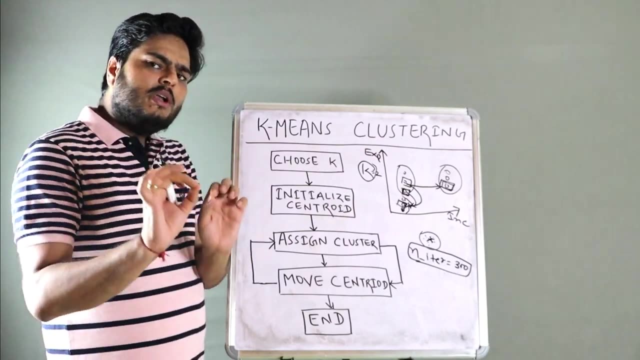 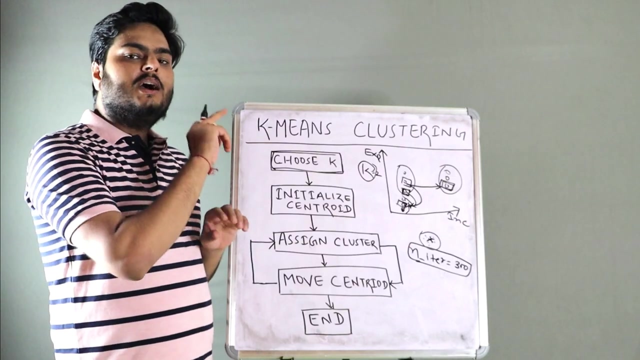 the new centroid, centroid and reassigning the data points. see here: reassignment, move centroid, reassignment, move centroid, reassignment, move centroid and finally converge. converge means if the centroid is not changing, that is nothing but convergence. okay, now one important question, guys: how to choose this k? okay, this is also an interview question. i will discuss about this in detail in my next video. 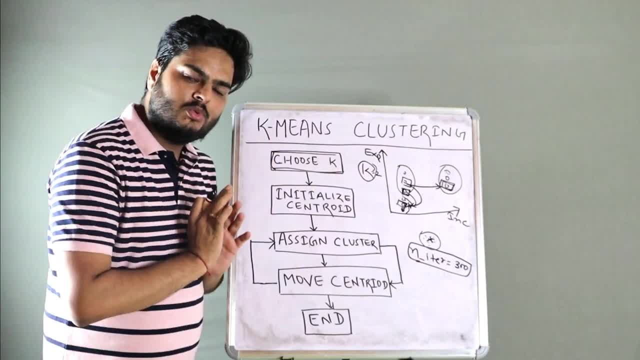 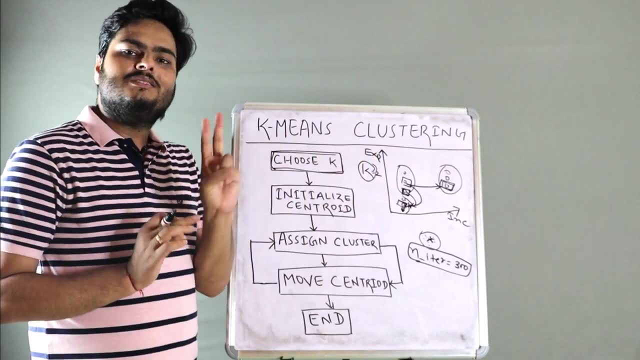 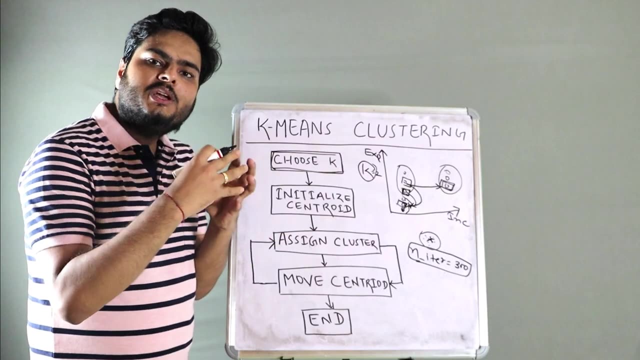 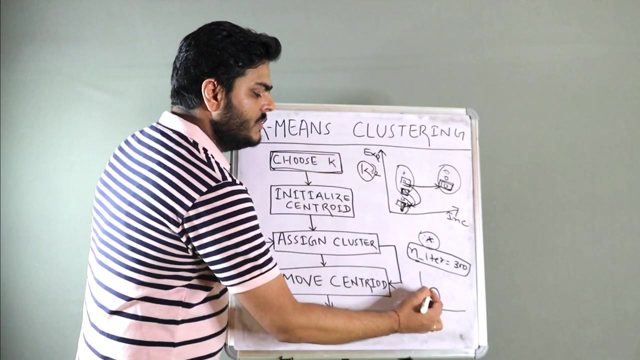 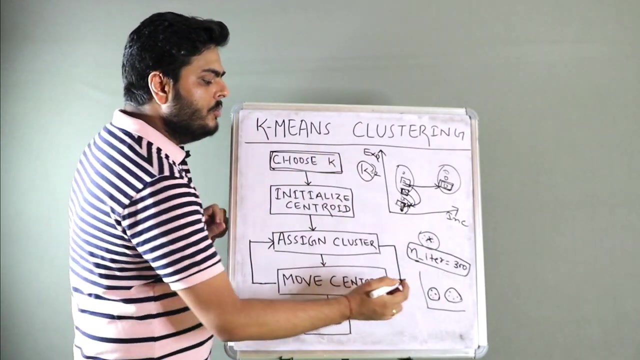 but for now, i am going to give you some idea. i am going to give you some idea about what centroid means. so let's 続 to 5. 5, 5, 3, 3, 3, 3, 3, 2, 2, 3. 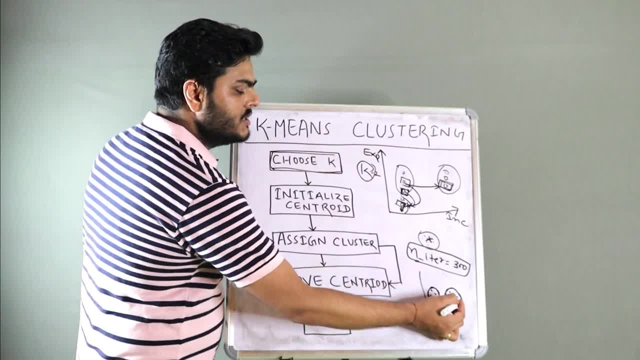 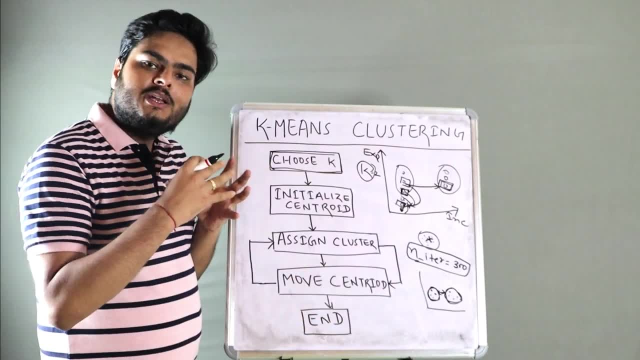 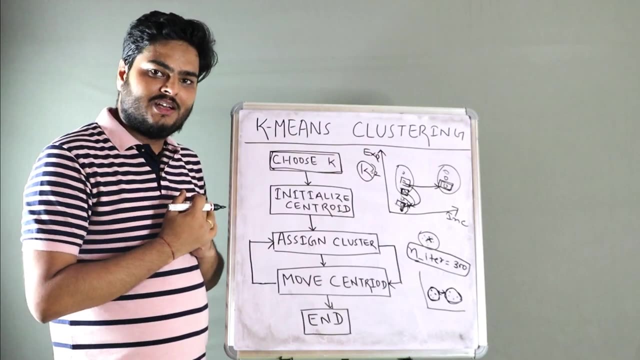 2, 1 and distance between the clusters should be far, which means two clusters should not be close to each other and points within the cluster should be near to each other. okay, how do we measure that points within the cluster are near to each other? how do we measure that? what we do is we just take 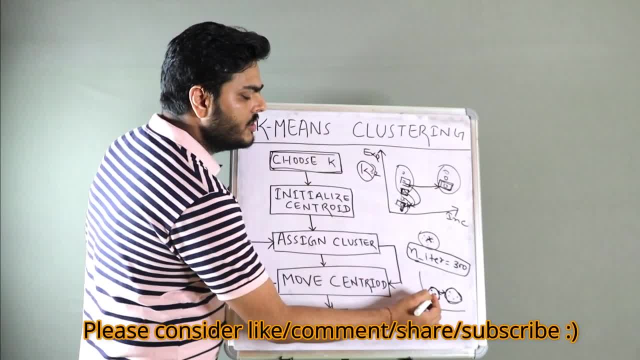 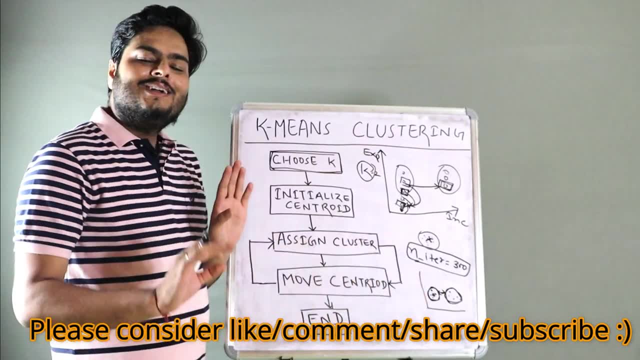 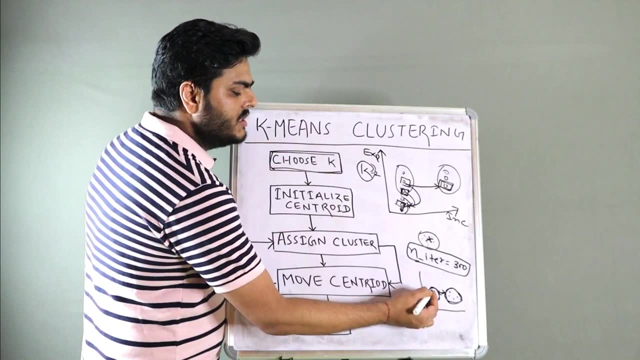 the distance of all these from their centroid. when i say distance, again euclidean distance, you can think of. okay, now let us say there are five data points. take all the, for example. there are one, two, three, four data points. this is centroid. all these four points. what is the distance from the centroid? 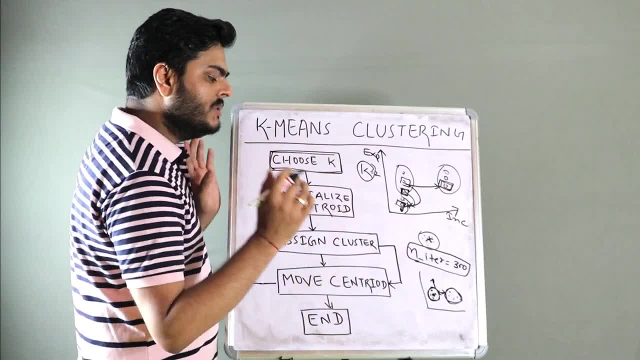 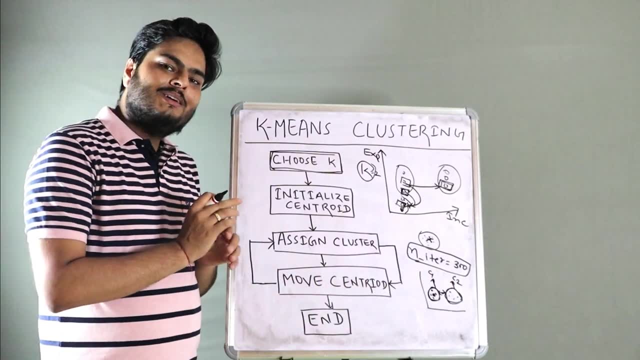 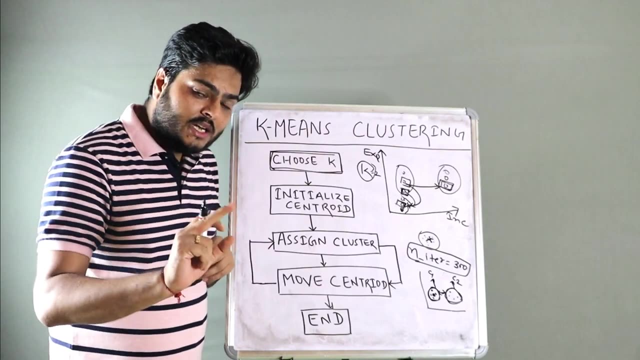 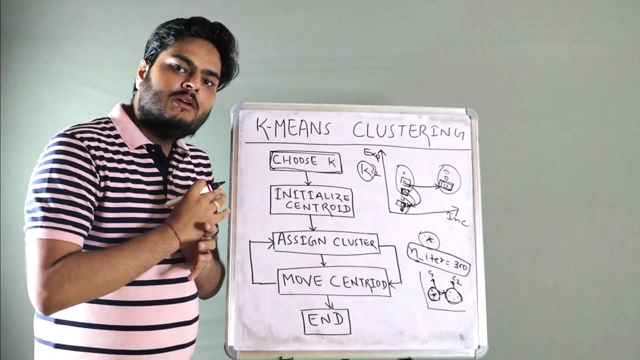 euclidean distance, that becomes the distance. sum it up, that becomes the distance of cluster. one same thing for cluster two. when you sum it up for all the clusters, right, that number is called inertia, or within cluster sum of squares. our objective, objective, objective, was to minimize that. minimize that, i told. within cluster distance should be minimum right now. 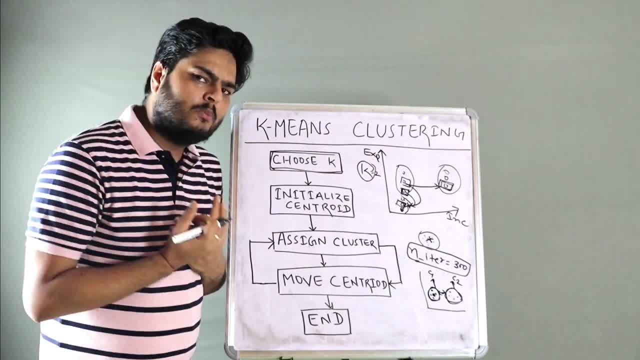 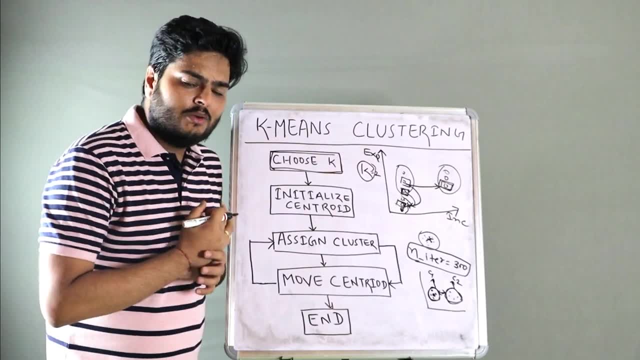 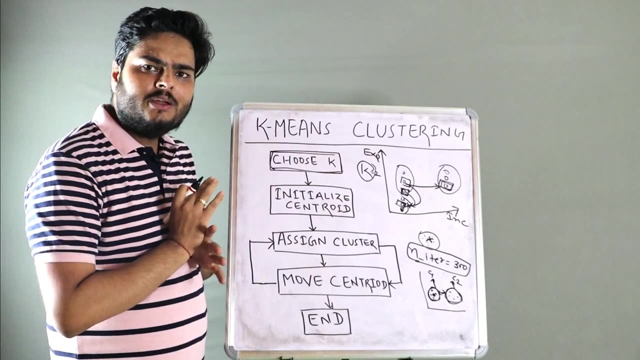 to choose k. one method that is very popular and everybody talks is known as elbow method. what we do is, since we don't know how, what is our optimal k? whether it is 2, 3, 4, 5, 6? we don't know. what we do is we roughly take a range of, let's say, 1 to 10? okay, and we see. what is this inertia? 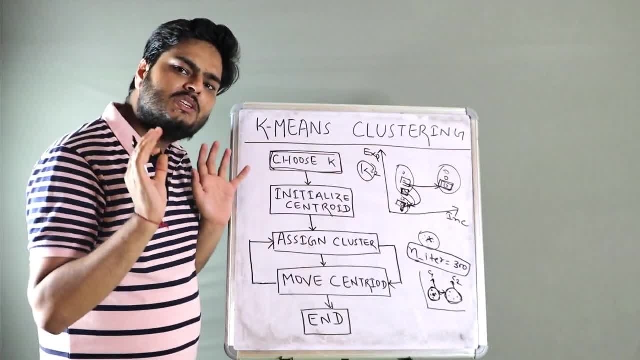 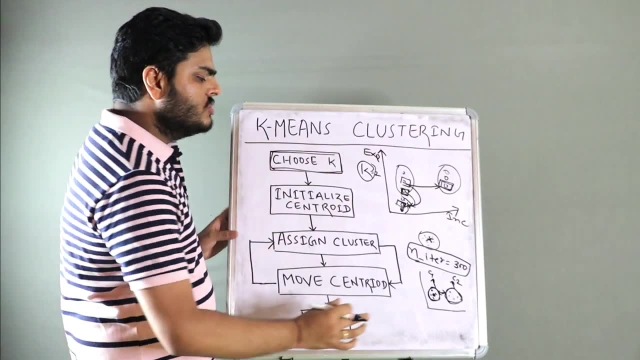 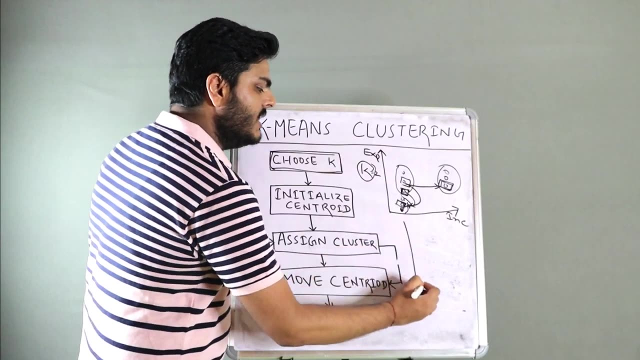 for example, when i have two clusters, then what is the inertia of all my clusters? when i have three clusters, what is the inertia when i have four clusters? what is the inertia? so what you will see is- i am just going to plot this here quickly- what you will see is a x- y chart like this: 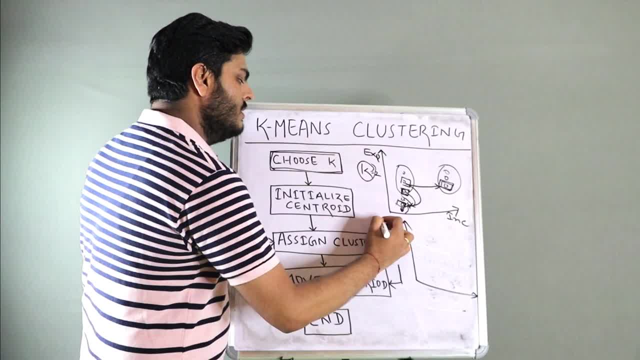 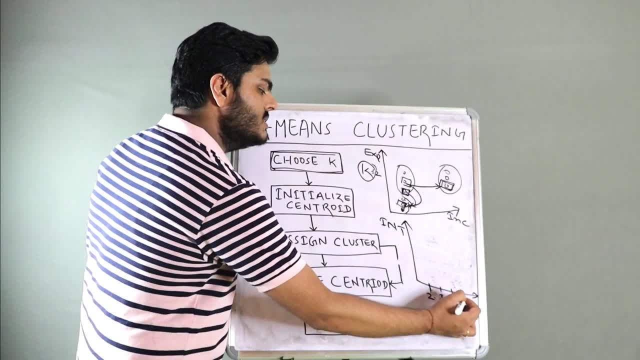 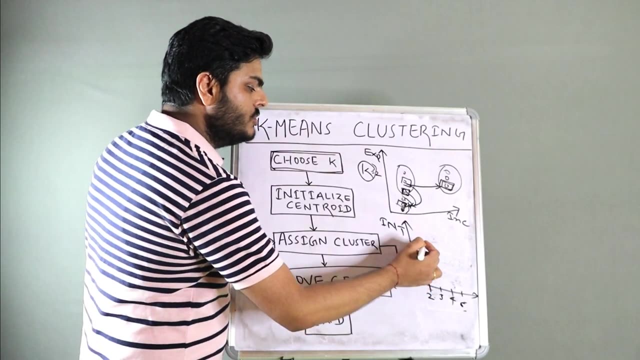 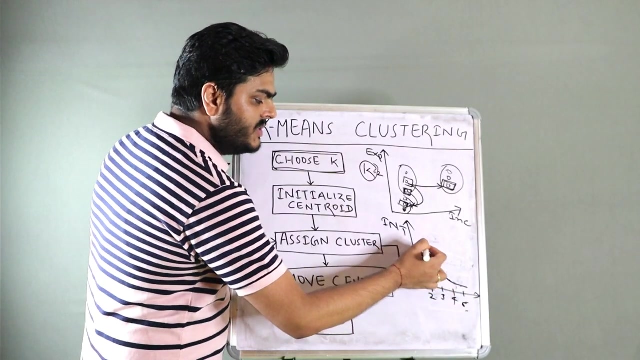 on one axis you will have inertia, okay, inertia, and here you will have value of k. so two clusters, three clusters, four clusters, five clusters. what is my value of inertia at all these clusters? so, for example, two is here, three might be here, four might be here, five might be here. so at the moment you see a steep decrease. this point becomes: 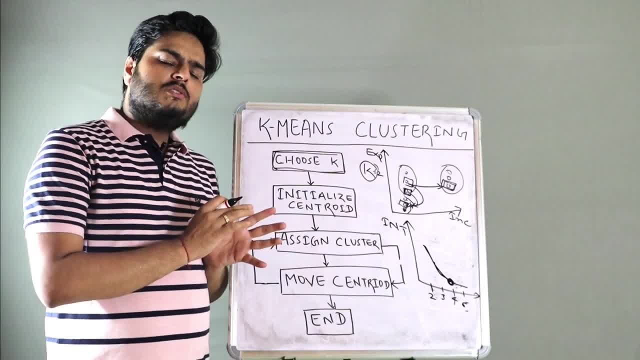 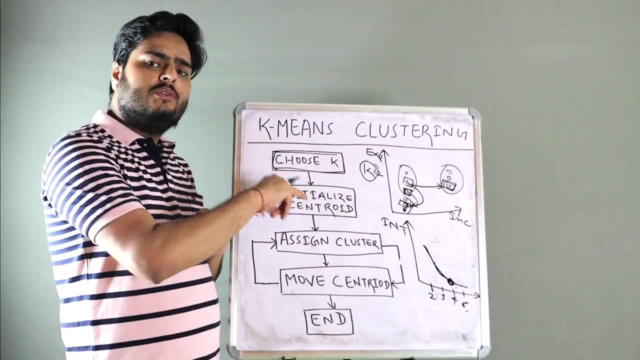 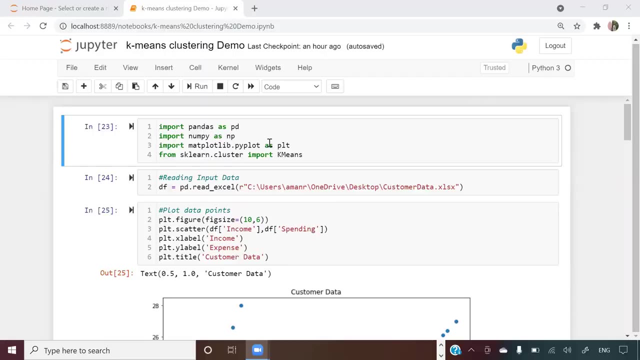 your optimal number of clusters? why? because we do not want to have many clusters. also, there are things around this which i will discuss in the next video. guys, there are interview questions around this. okay, before that, let me show you how to do the same thing in python. let's see in my screen, hey guys. so here one simple example. right, uh, i'm 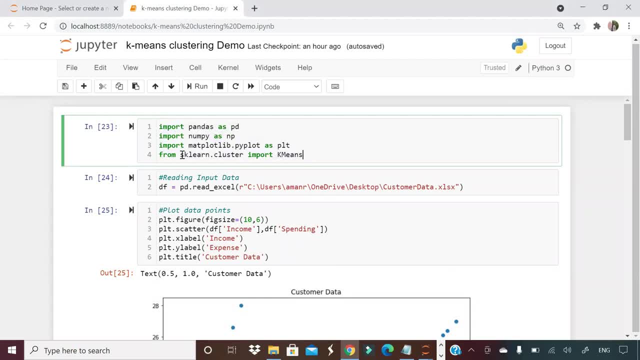 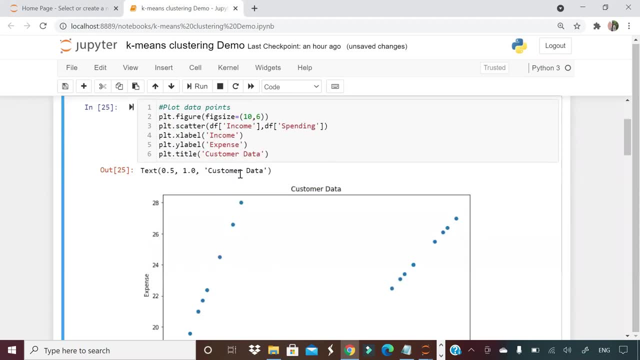 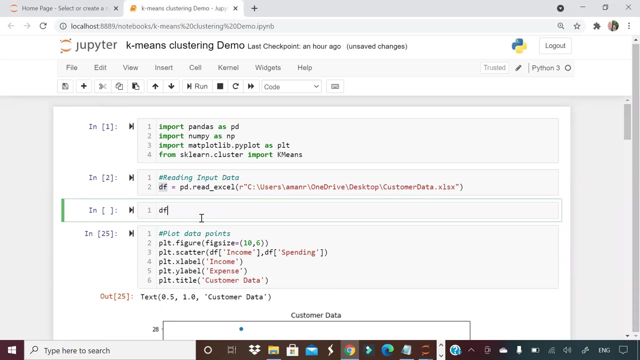 importing some of the packages here and if you can see, i'm importing from sklearncluster, import kmeans. okay now, kmeans, we will be implementing. i have a simple data here, df. i'm reading that and let me show you head of df so that it becomes easier for you. and then i'm obviously 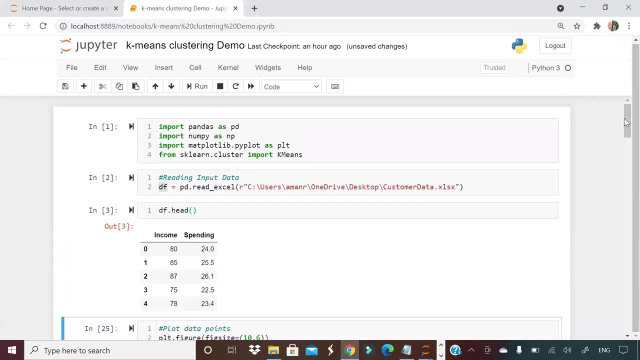 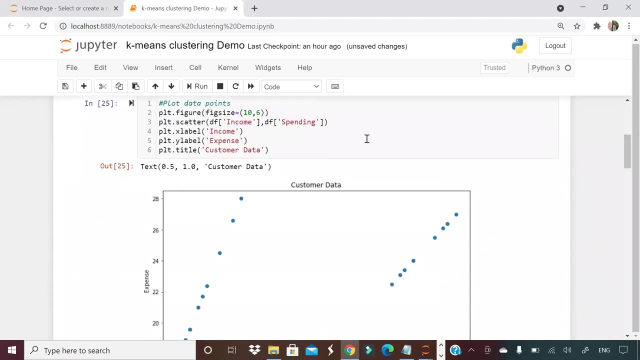 plotting df below, so dfhead. same kind of data that i was explaining you, just two columns: income and spending. okay, and i have created a data to demonstrate you in such a way that there are people i have plotted the same data. okay, there are people who are earning less. 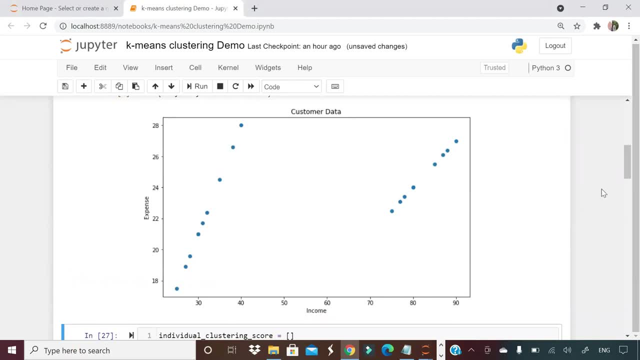 but spending little higher. there are people who are earning little more, but you know spending in the similar range. so savers and aggressive spenders. you can say now the first thing we choose, k right. so as i was telling you, there is an elbow method for that, what i'm doing. 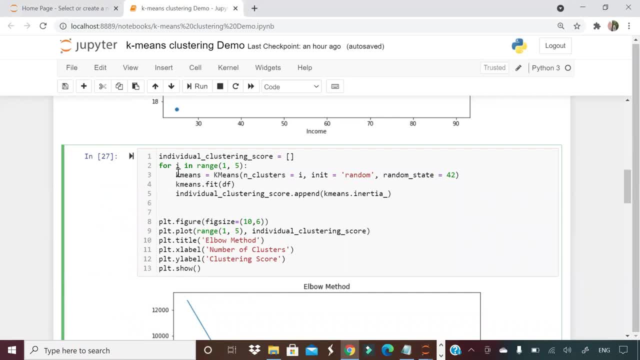 here is: i don't know what is my optimal k. so i'm running five k means model here. if you can see, i'm saying for i in range one to five k means is equal to number of clusters, is i which is in for loop, and then i'm passing my data. 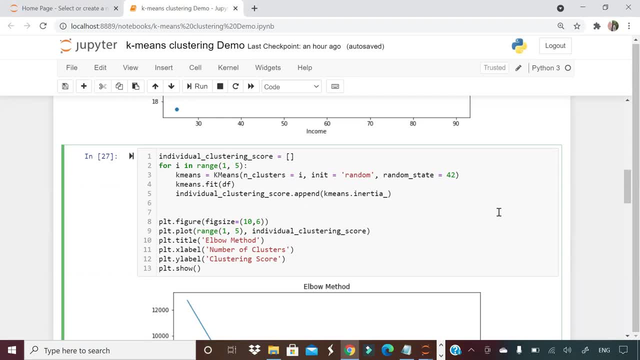 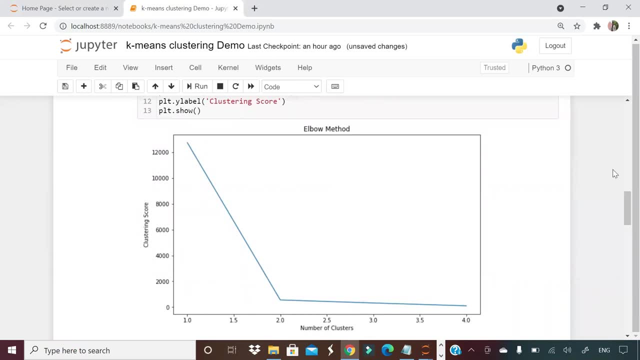 tf. right, i'm appending all this score and i'm getting a elbow curve like this. now, if you see this, elbow guys, this is nothing but clustering score, or what i was telling you is inertia. if you see, here i'm taking inertia. k means dot inertia. inertia is nothing but. 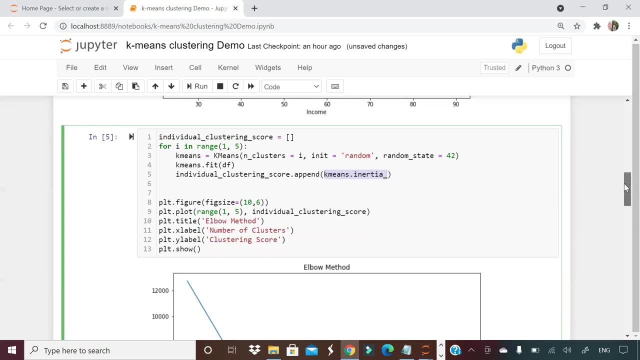 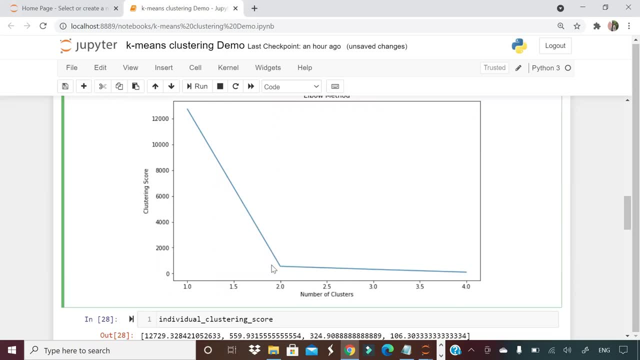 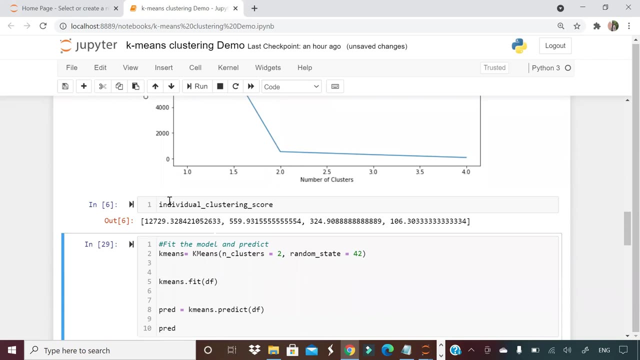 within cluster sum of squares. okay, it will reduce with increase in k. okay, but i told you, whenever there is a steep decline, that becomes our optimal k. so in this case, two is our optimal k. so how inertia is changing. if you want to see, you can just see here individual clustering score. i have put in this list, right. 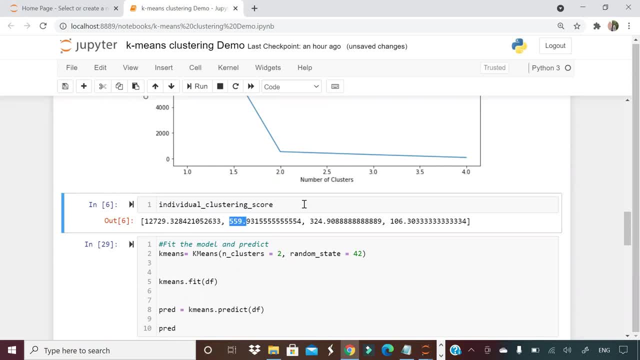 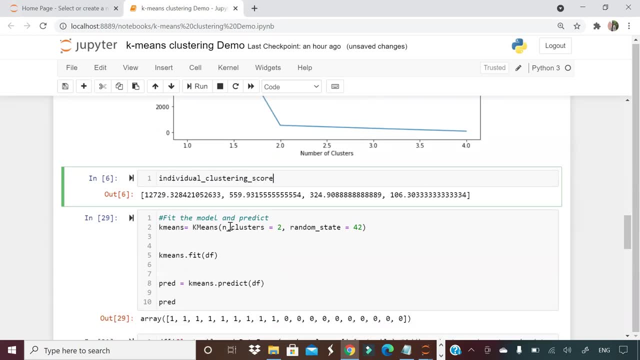 so previously it was 12k, now it became 559 suddenly. so a huge shift, right. that is why i am taking as two. now i am considering that two. i am saying k means model is equal to number of clusters. is two fit on df and predict also what is my cluster number. so, as you can, 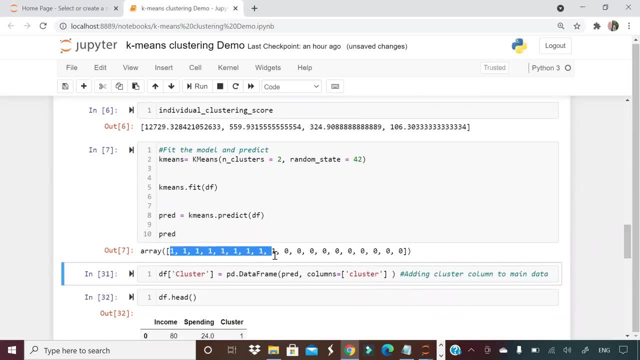 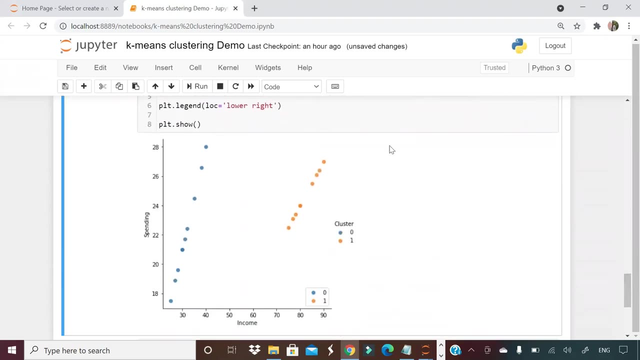 see it is predicting first 10 observations in cluster one and next 10 observations in cluster 0, two different clusters. i will take this data and i will, you know, paste this as a column in the df itself. now df looks like this and i am plotting the df again with different.